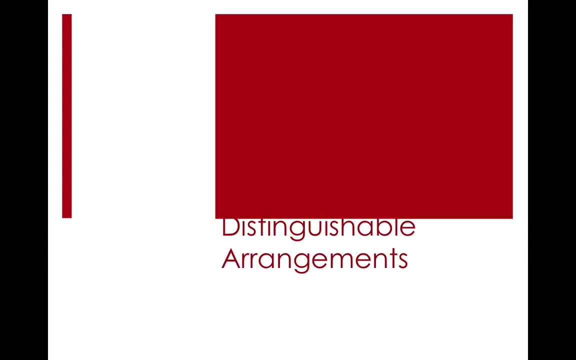 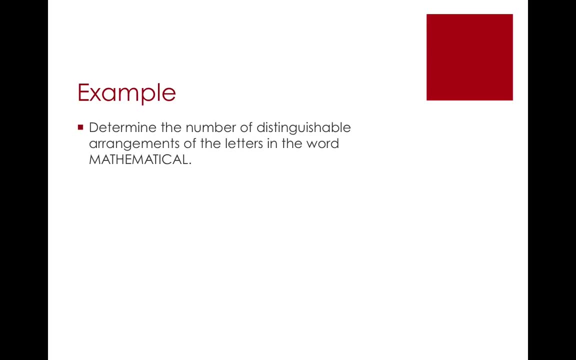 Distinguishable arrangements. In these problems we're going to have to try to distinguish or tell the difference between different items. So we want to determine the number of distinguishable arrangements of the letters in the word mathematical. So what we mean by distinguishable is some: 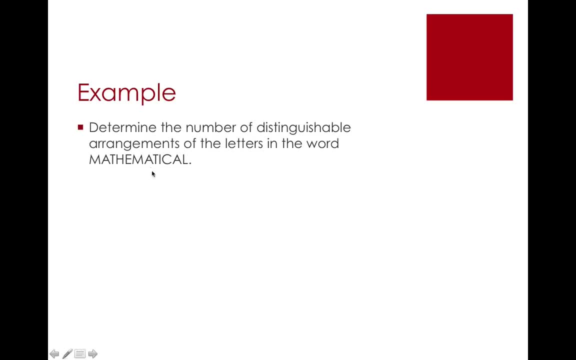 of these letters are identical, For instance the A's. If I were to just switch the A's and no other letters, I couldn't distinguish this from the original problem. But if I were to switch the A and the L, for instance, then I would know. it's a new word, One way. 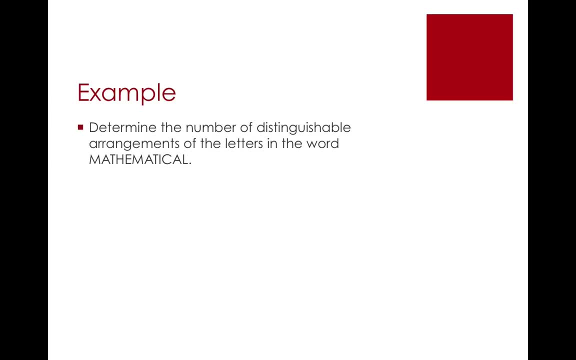 to think about. it is Scrabble tiles, So each letter is on an individual tile. I wouldn't know which A I picked out, if it was this A, this A or the last A. They all look exactly the same. So this is how the problem works. You take the total number of items In this. 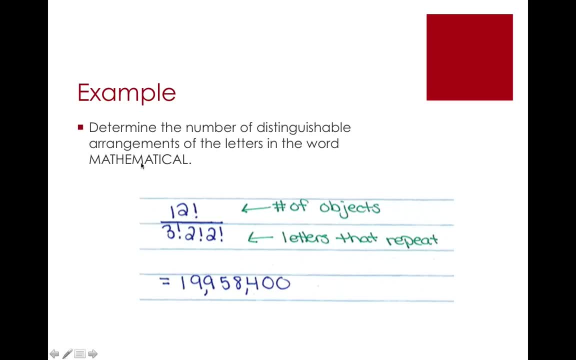 case there's 12 letters: 1,, 2,, 3,, 4,, 5,, 6,, 7,, 8,, 9,, 10,, 11,, 12. Factorial: You take the total number of items, divide it by the numbers that repeat. So there are 3 A's, that's. 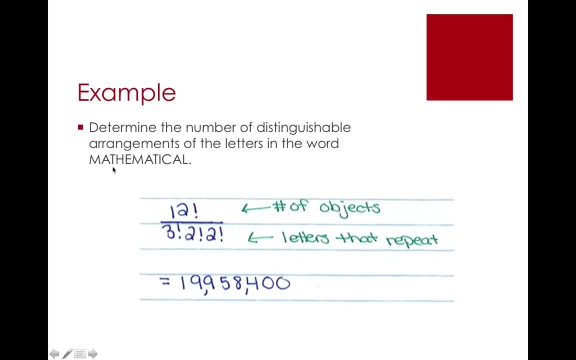 the 3 factorial, 2 M's and 2 T's. Now when you type this in the calculator, you either need to split it up into steps- type in the numerator, get an answer. denominator- get an answer and then divide, Or you need to put parentheses around the denominator. so 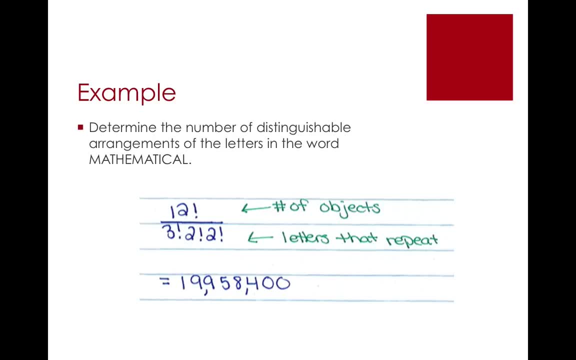 that the calculator knows. all of those numbers are in the bottom. Let's look at another problem: Determine the number of distinguishable arrangements of the letters in the word mathematical. The number of distinguishable arrangements of eating a package of Skittles with 4 red. 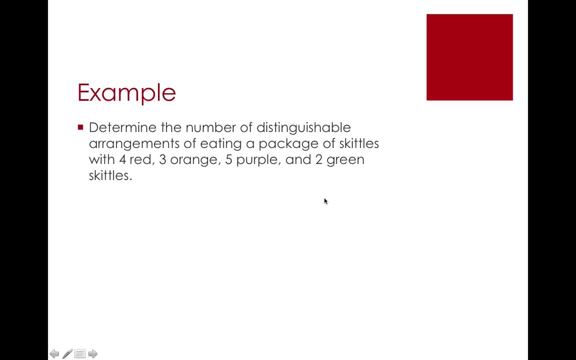 3 orange, 5 purple and 2 green Skittles. Again, if I put out a green Skittle, I wouldn't know which of the two it is- They would look exactly the same. Total: there are 14 different. 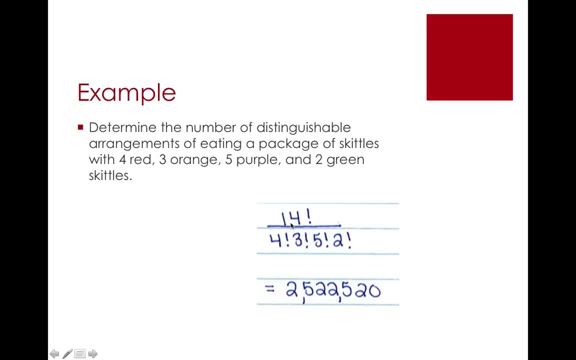 Skittles: 4 plus 3 plus 5 plus 2, 14 Skittles: 4 reds, 3 orange, 5 purple, 2 greens. Those are all my repeats and they get factorials as well. Remember the factorial button is. 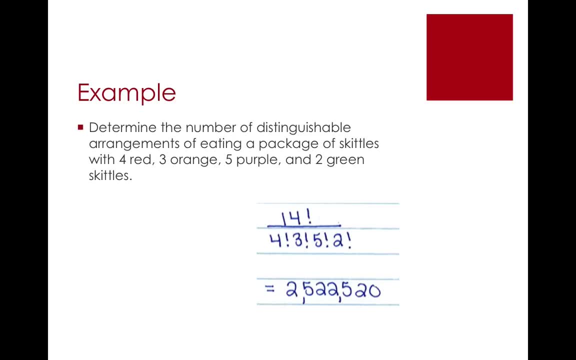 on your side your calculator, or you can type in what it is out by hand. It's whatever the number is, multiply by everything less than that. So 4 times 3 times 2 times 1 is 4 factorial.